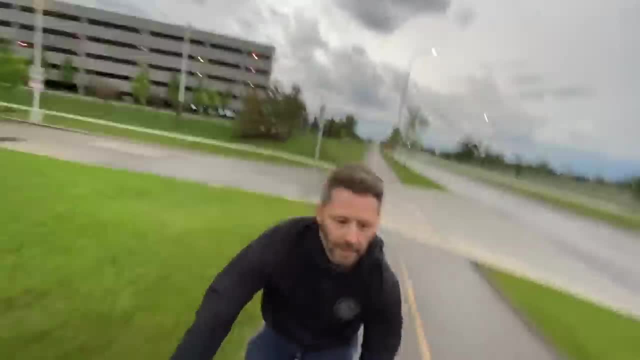 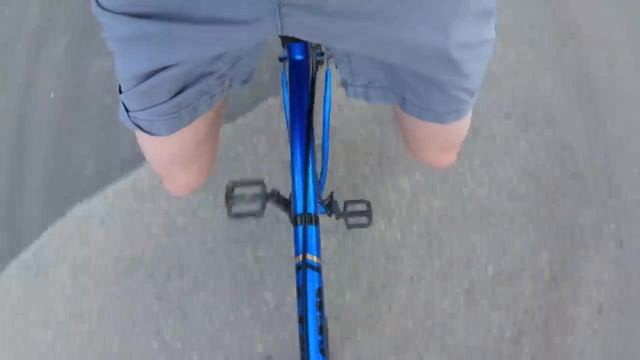 newbies on Fixies to do normal things like hop a curb or like descend a hill without going crazy. I mean, when you go down the hill the pedals are going like crazy. I actually found myself taking my feet off the pedals and just letting it. 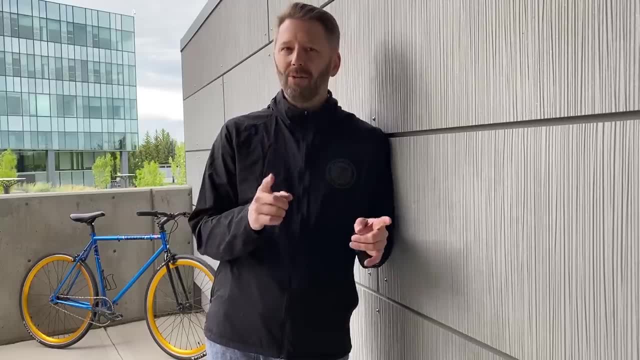 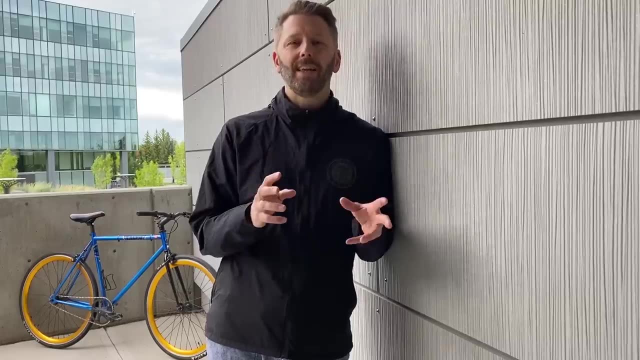 roll, which is kind of absurd when you think about it. But there are a few things about the Fixie that I did kind of start to maybe appreciate. Here's my new thing: Fixies are ridiculous, except for three things. Okay, the first one came. 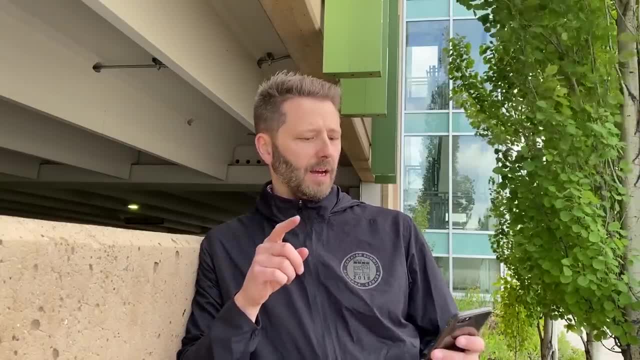 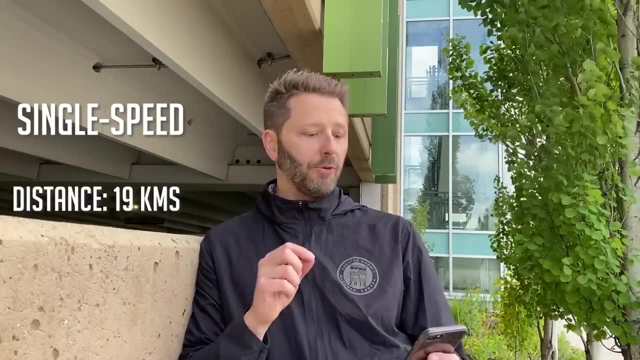 to me when I was recording my commutes. Now this is what I got On the single speed. if I combined the morning and evening commute, I rode for 19 kilometers for a time of 54 minutes 19 seconds, with an average speed of 21.05 kilometers per. 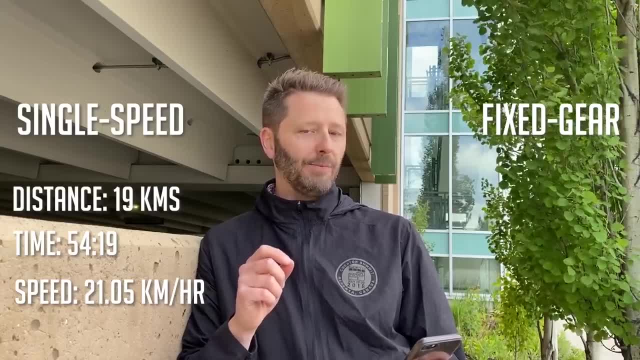 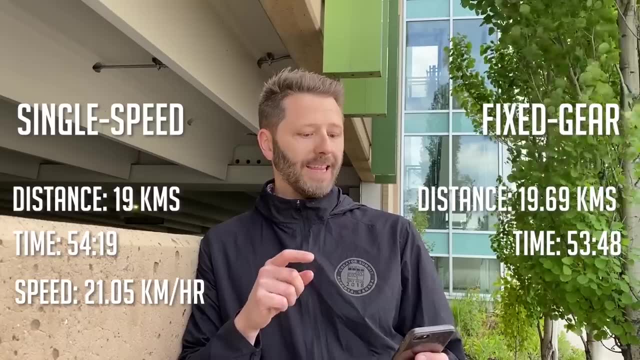 hour On the Fixie. I rode 19.69 kilometers in 53 minutes 48 seconds, for an average speed of 21.65 kilometers an hour. So yes, the Fixie is faster. This is the second time I've done this kind of thing. 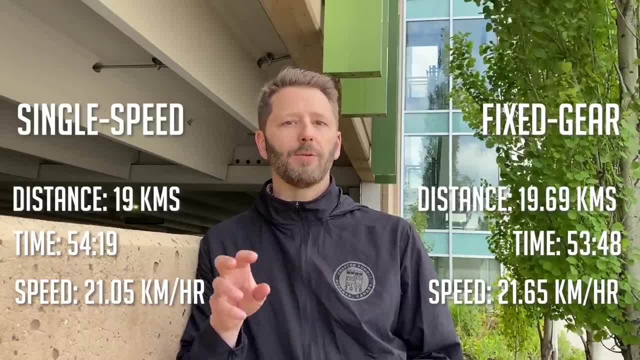 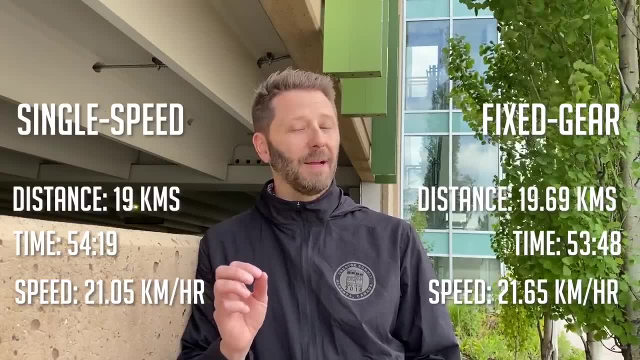 Earlier I did a challenge where I commuted on a Fixie, a single speed and a road bike and in that case the Fixie was also faster. You know, not by much in this time, but I do feel like when I'm riding the Fixie I am going faster than the 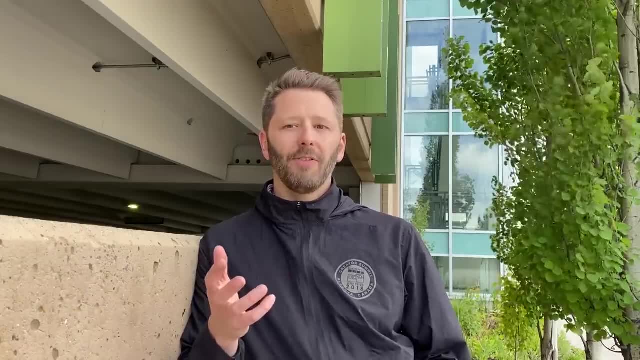 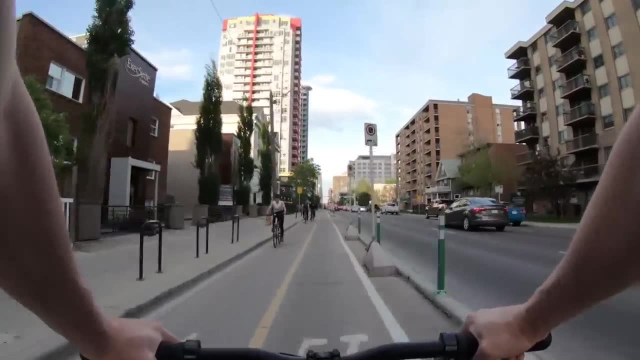 single speed, which is kind of unexpected, I think, And I think it's because of the momentum of the drivetrain. because you can't coast, Pedals are always nudging you to go faster and faster, to keep pedaling and keep pedaling. Psychologically, or maybe a little bit physically, the bike does. 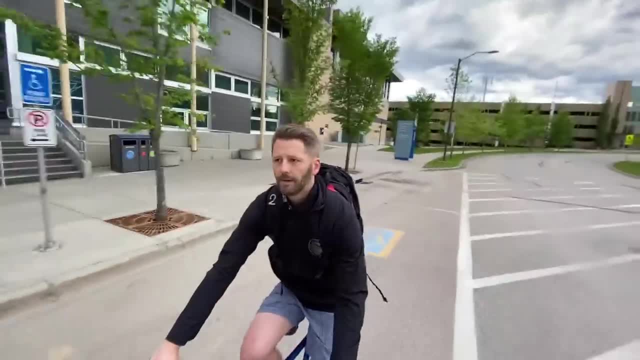 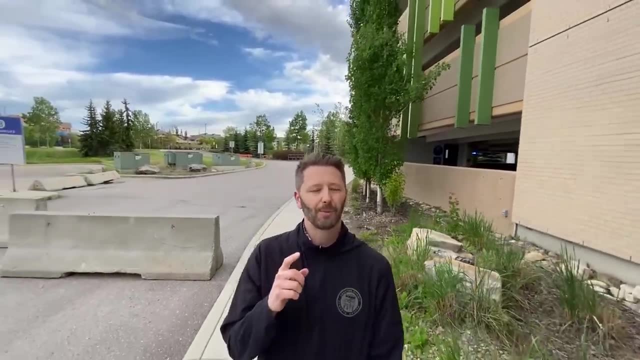 compel you to go a little bit faster than the single speed. So yeah, who knew The Fixie is faster? Just a little bit, but still faster. That brings me to the second point that I'm maybe starting to appreciate about the Fixie, and that's: 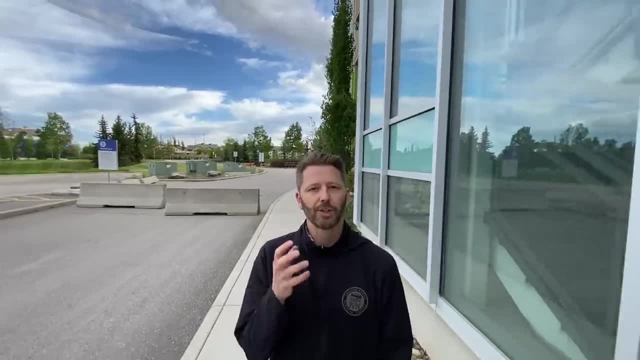 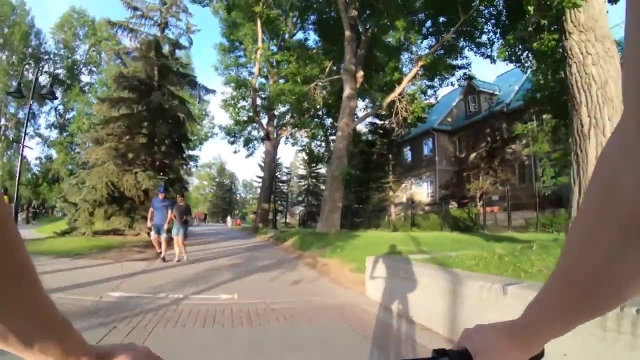 the control. So those in the Fixie cult are always talking about the control that that fixed gear drive gives you. You can really feel the asphalt, they say, or you can feel the bike better than ever before. It gives you more control And I never really understood that. 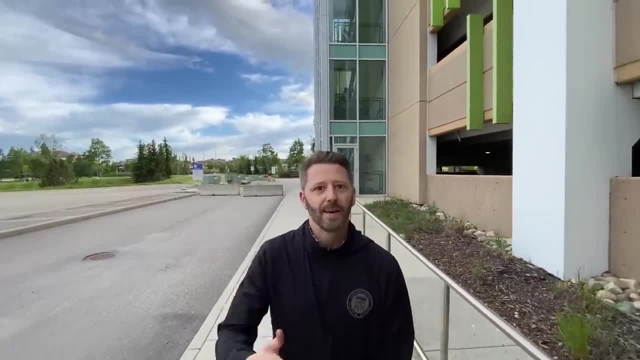 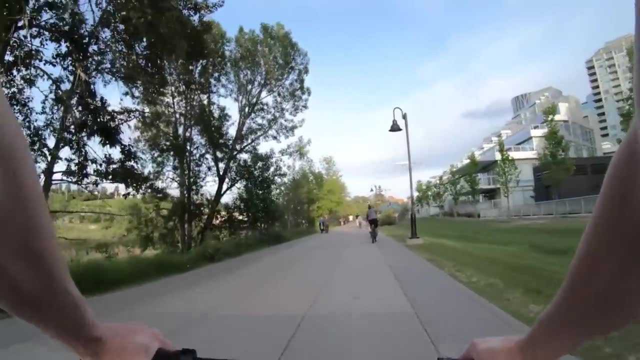 because I was always worried about getting tossed off the bike because those pedals would just never stop When I think about it. you know, whenever you see someone doing a track, stand at a red light or riding a bike on a tightrope dressed as a clown, they're usually riding a Fixie. And I'm starting to.